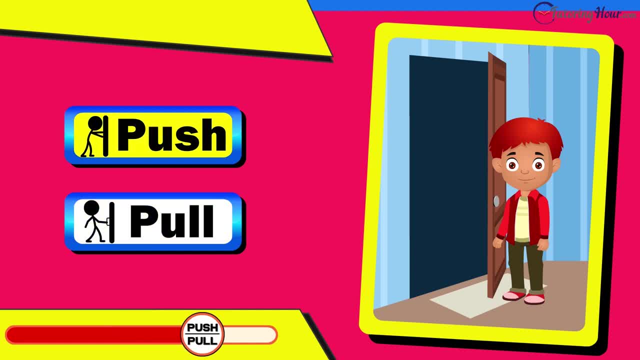 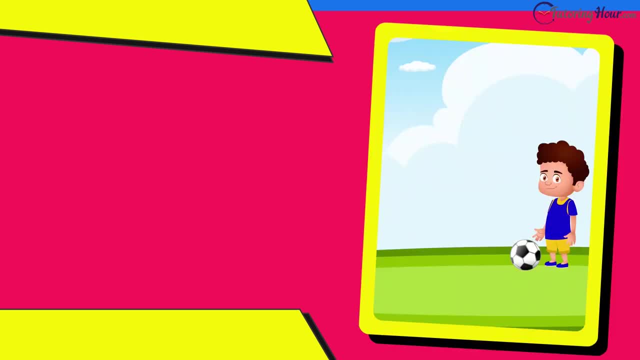 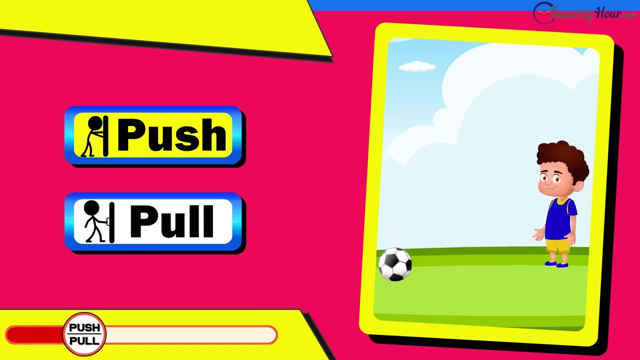 The correct answer is a pull force. Let's move on to the next question. What force is exerted when you kick a ball forward? Is it a push or pull? The correct answer is push force. When you tug on the rope to lift a bucket from the well, what force are you using? 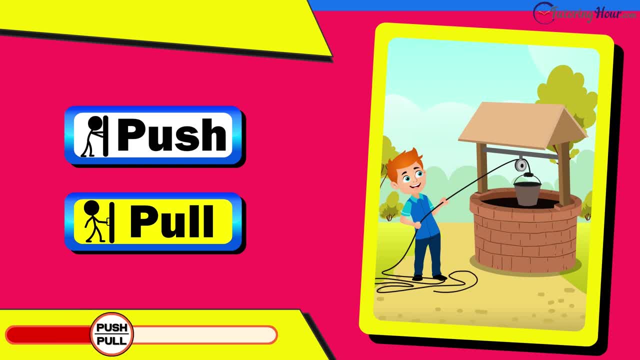 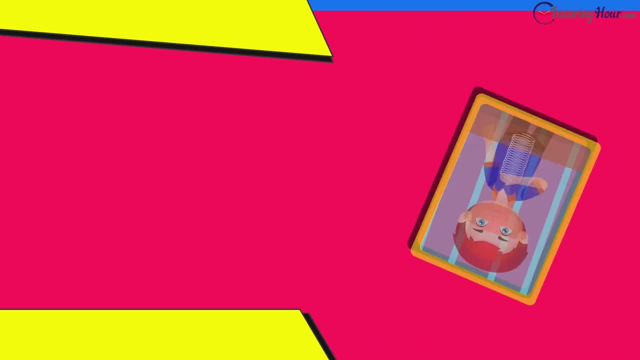 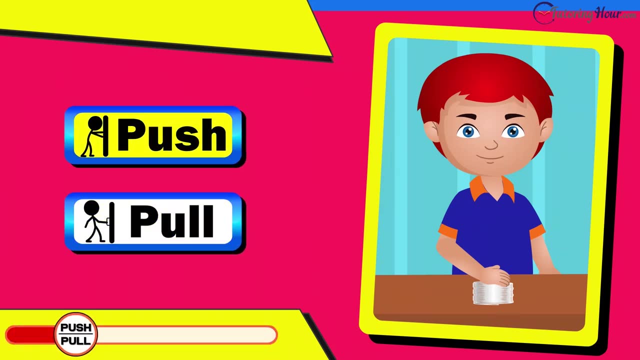 Is it a push or pull? The correct answer is pull force. When you compress a spring, what force are you applying? Is it a push or pull? The correct answer is push force. What force is used when you draw a bowstring to shoot an arrow? 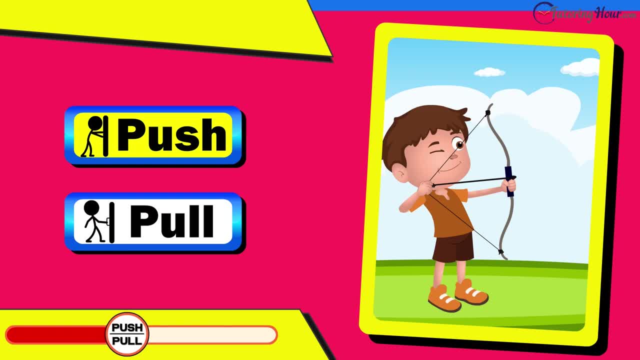 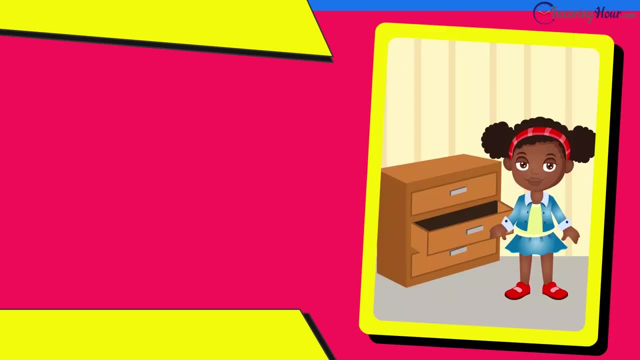 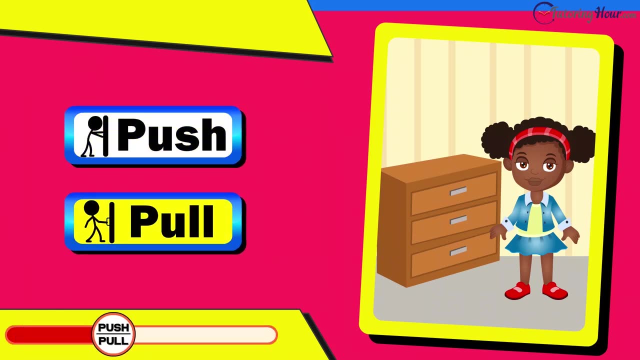 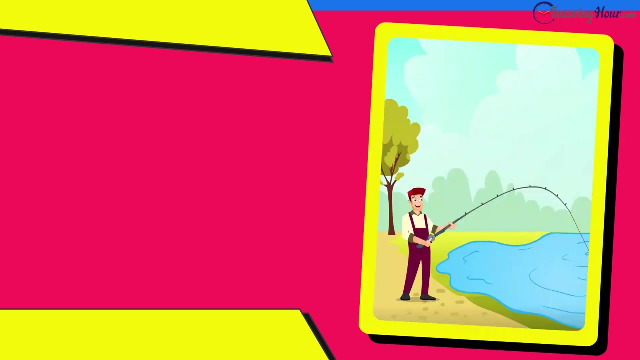 Is it a push or pull? The correct answer is pull force. When you close a drawer, what force are you using? Is it a push or pull? The correct answer is push force. When you reel in a fishing line, what force are you exerting? Is it a push or pull? 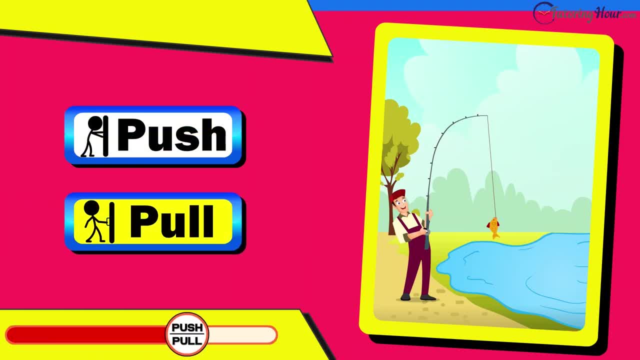 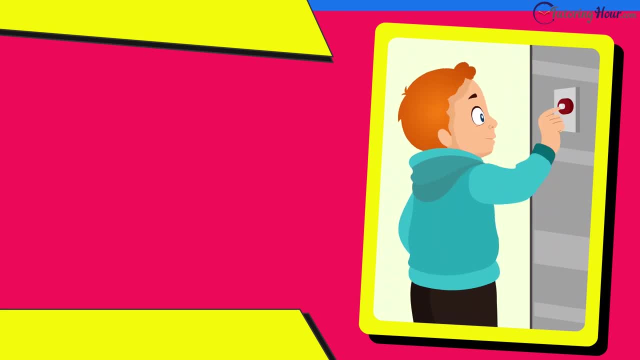 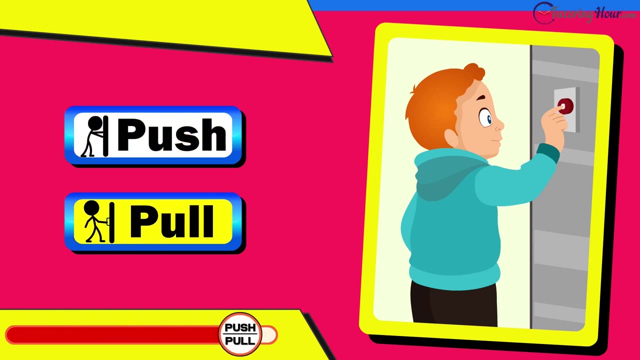 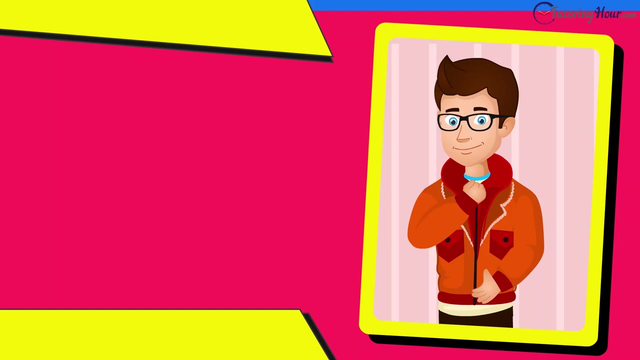 The correct answer is: pull force. What force is exerted when you press a doorbell button? Is it a push or pull? The correct answer is push force. When you are zipping your jacket, what force are you using? Is it a push or pull? 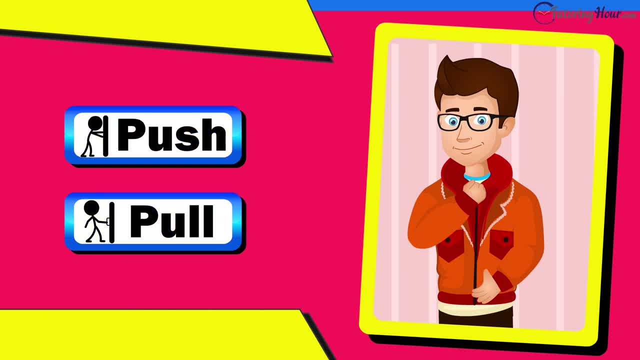 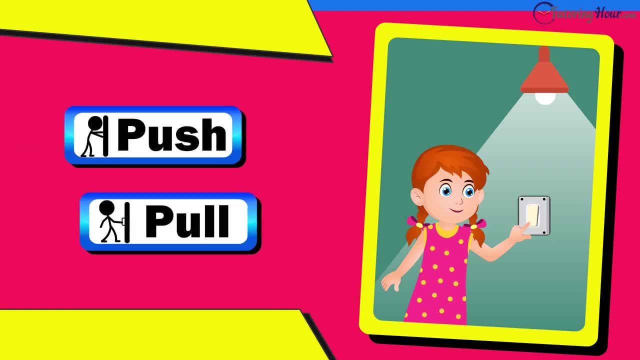 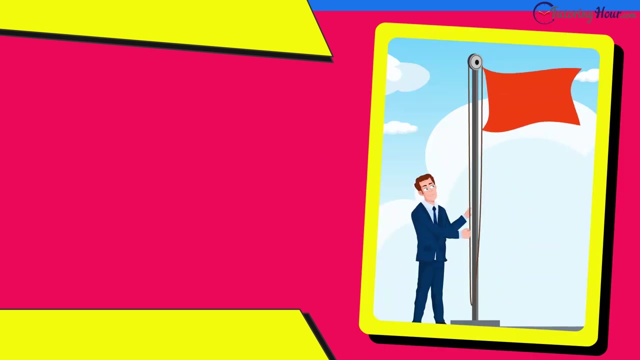 The correct answer is pull force. What force are you using when you turn on a light? Is it a push or pull? The correct answer is push force. When you are hoisting a flag up, what force are you using? Is it a push or pull? 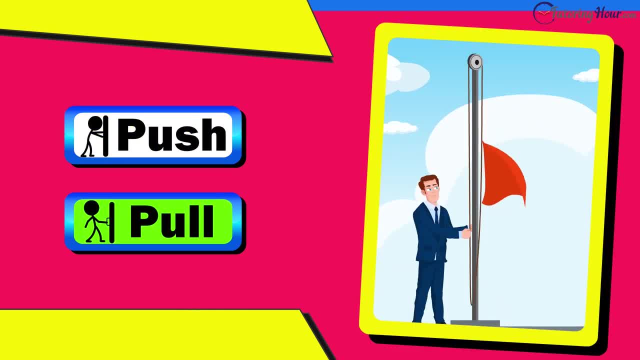 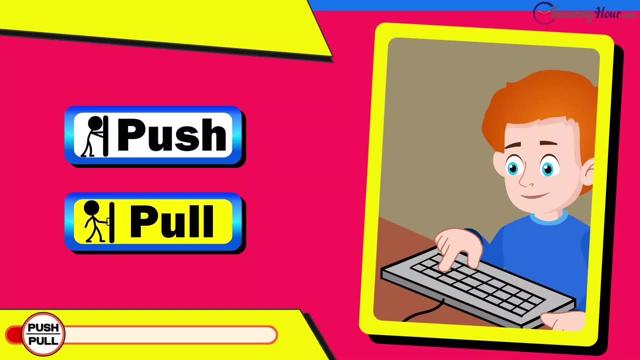 The correct answer is pull force. When you press a key on a keyboard, what force are you using? Is it a push or pull? The correct answer is push force. What force is used when you drag a heavy suitcase? Is it a push or pull? 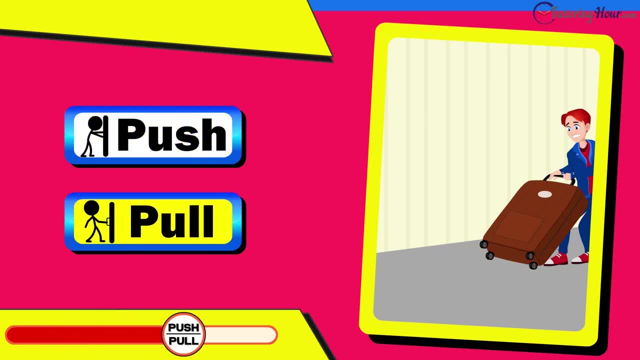